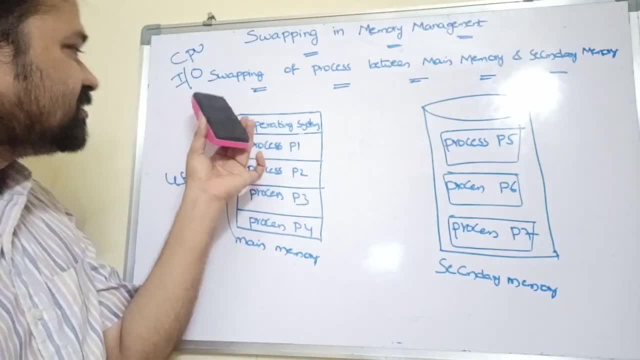 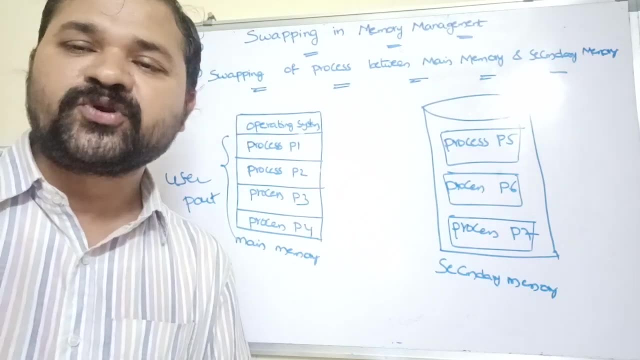 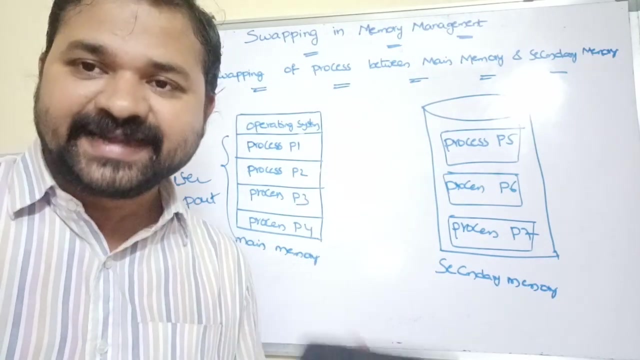 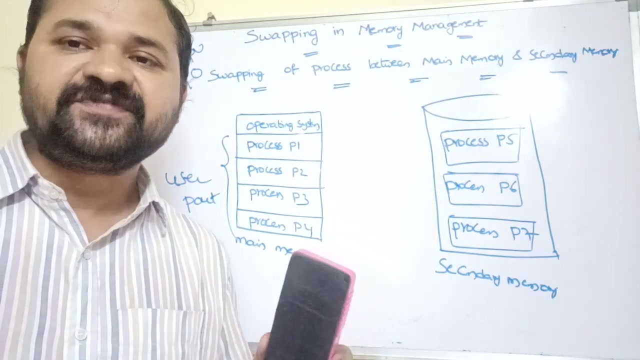 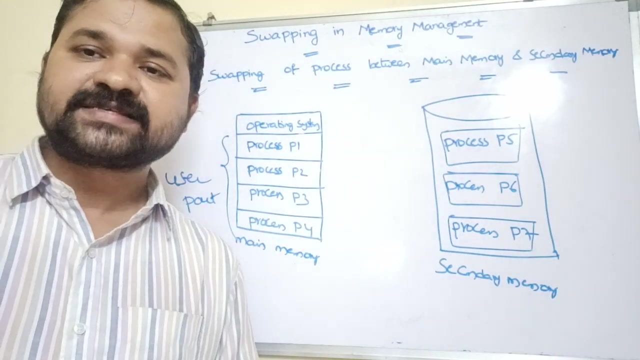 dead slow. I stands for input operation, whereas O stands for output operations. Input operations mean reading some data, whereas the output operation means writing some data in operating system are needed for it. Meanwhile, in order to perform the operation, we can use read system or. 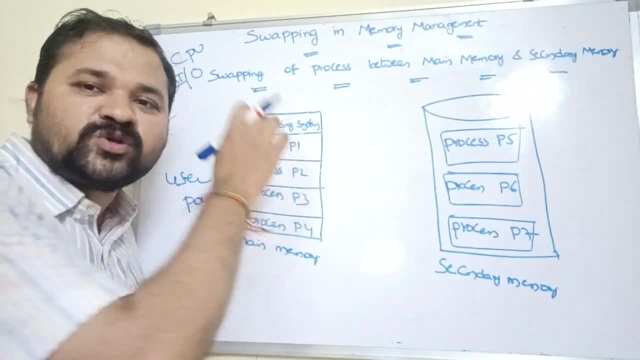 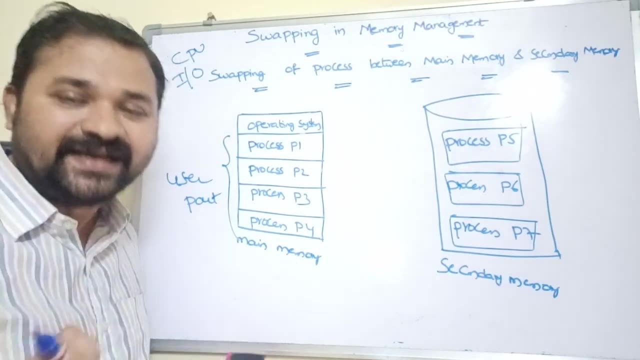 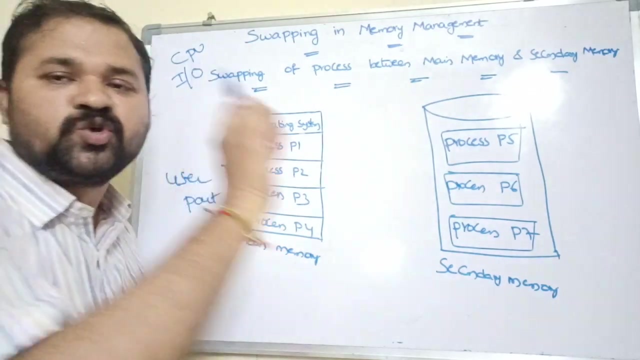 So here the point is. let us assume that process P1 is waiting for some Ivo operation. During Ivo operation CPU is idle. Why? Because CPU can't perform the Ivo operation. It is the responsibility of operating system to perform the Ivo operation. 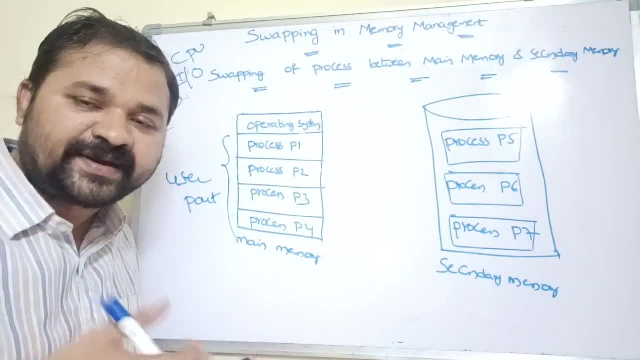 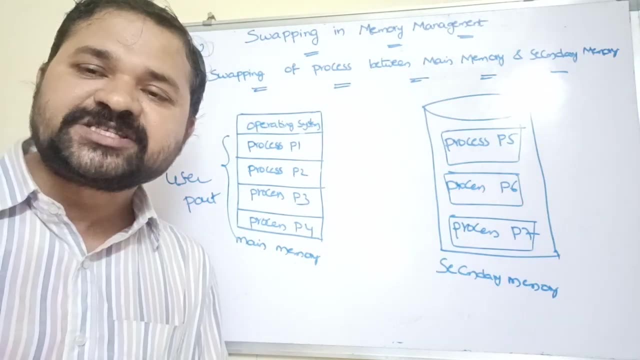 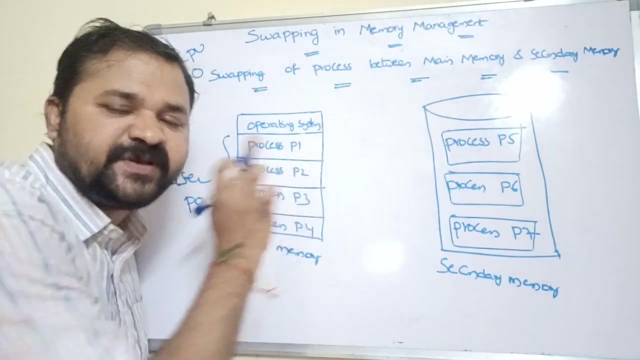 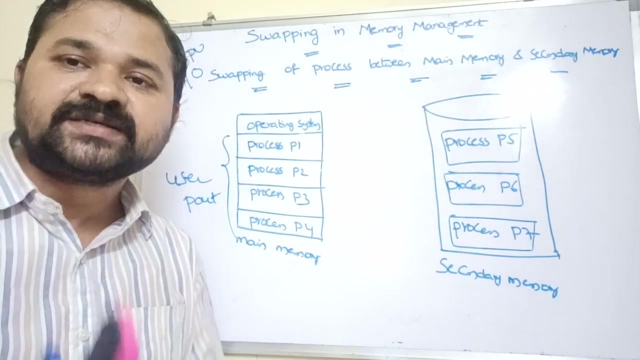 So while process P1 is waiting for some Ivo operation, then CPU is idle. So what the operating system will do is: operating system allocates the next process to CPU. So CPU starts executing process P2.. Let process P2 is waiting for some Ivo operation. So during that day CPU is idle. Why? Because CPU can't perform Ivo operation. 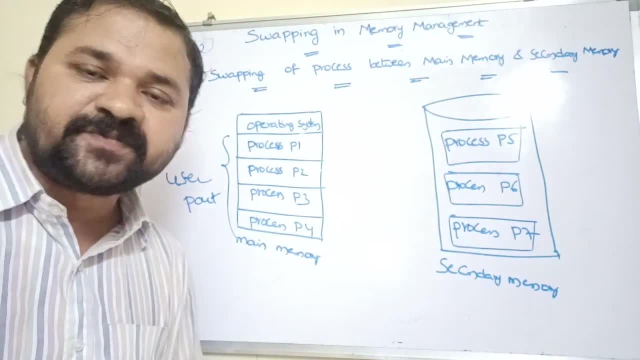 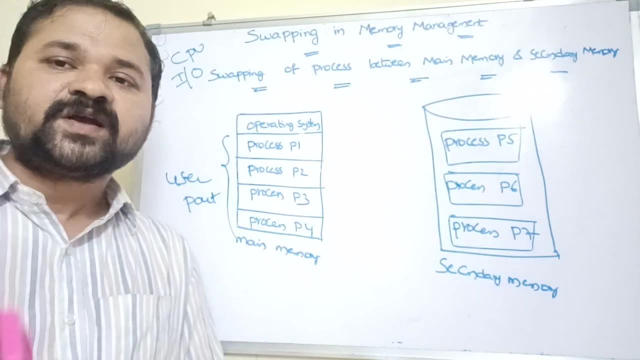 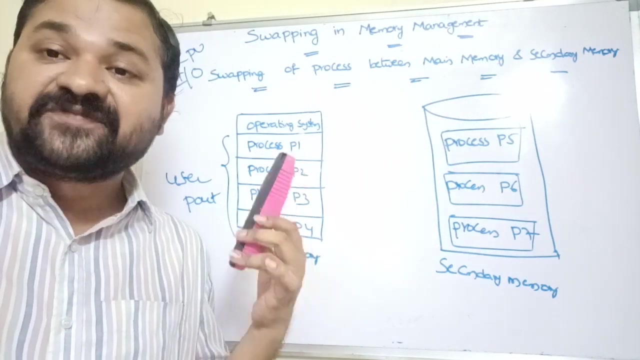 So what the operating system does, system will do. operating system allocates the next to process. that is nothing but process p3 to CPU. so in this way, most of the time, okay, the CPU is very, very busy, so we can utilize the efficiency of the CPU in effective. 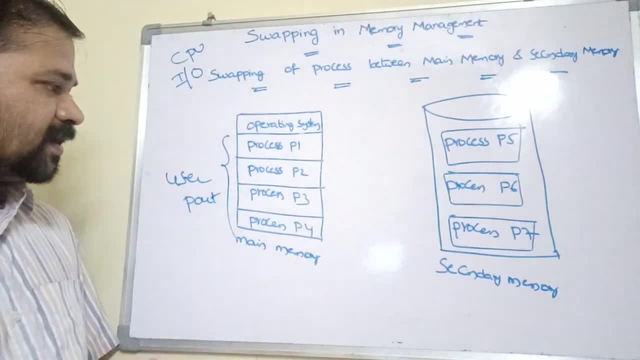 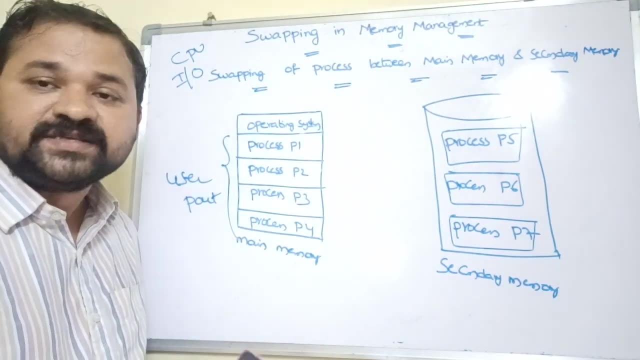 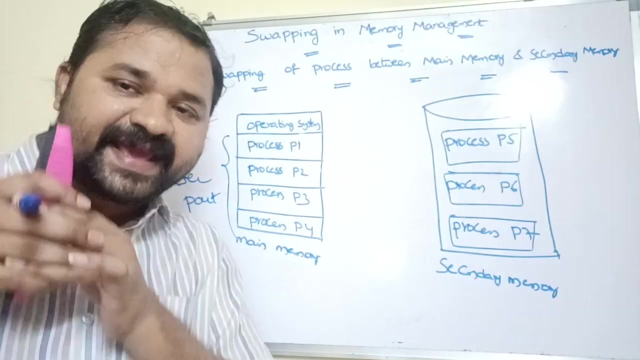 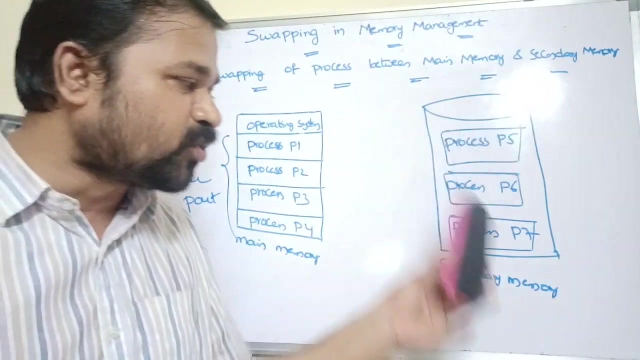 manner with the help of the multi programming system. here we know that CPU can access only the content of the main memory. CPU can't access the content of the secondary memory directly. so here CPU can execute a program or a process if it resides in main memory only. suppose if a process resides in. 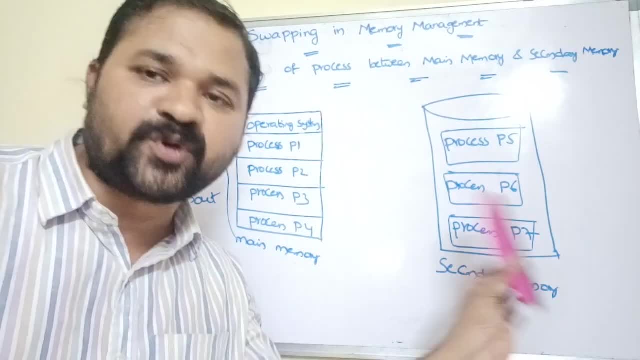 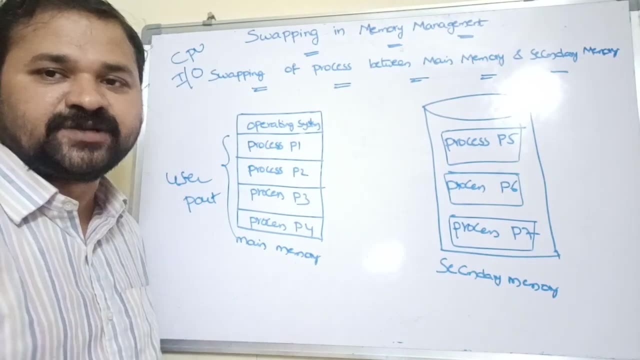 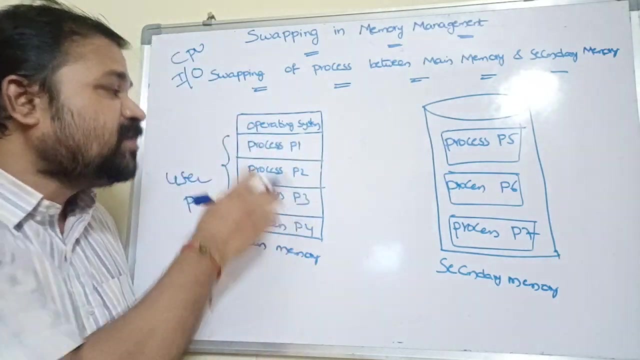 secondary memory, then CPU can't execute that process. okay, so here let us assume that process p1 has completed its execution. so that means process p1 completed all its operations. so now there is no need of CPU for process p1. so here what will happen is this process will be transferred. 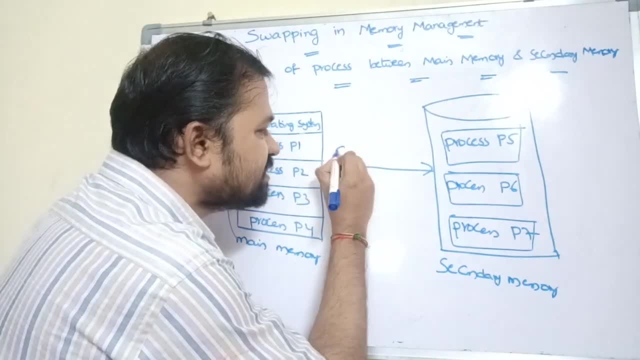 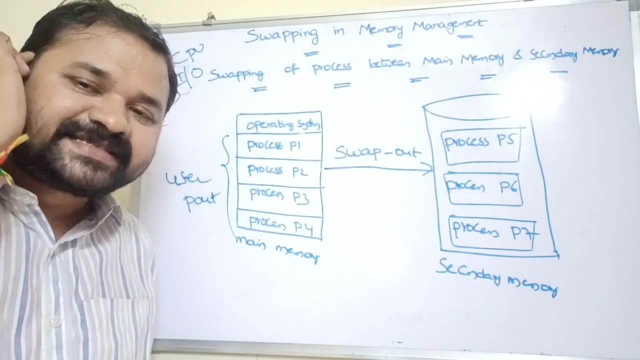 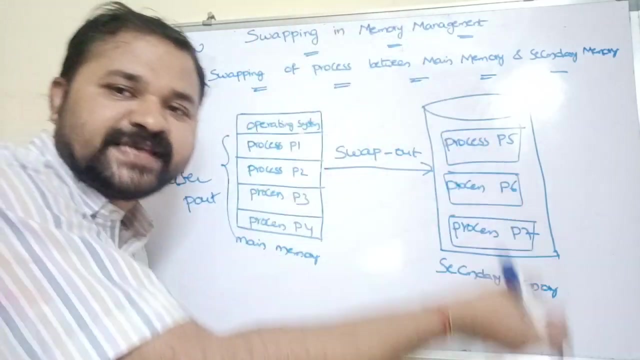 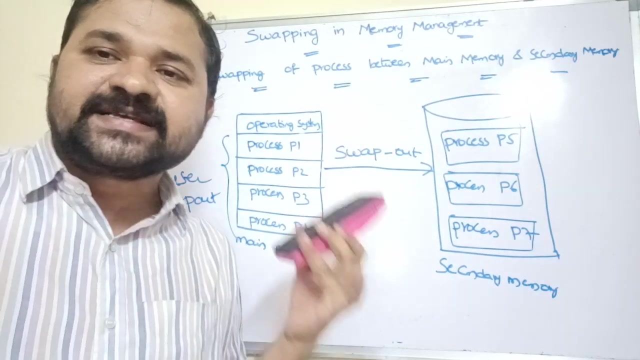 to the secondary memory. so this transferring is known as swap out. so whenever process p1 completes its execution, then operating system transfers process p1 from main memory to the secondary memory. so this process will be transferred to the secondary memory. so this transferring is known as swap out. there are various scenarios where the 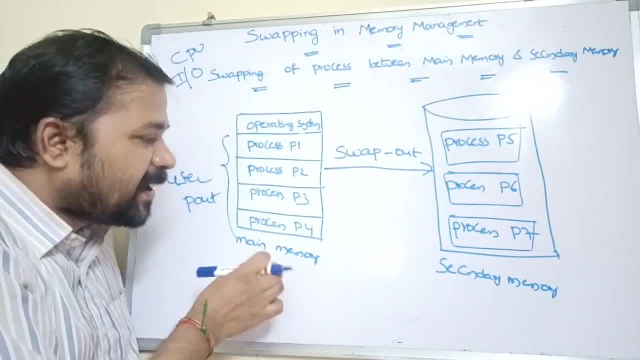 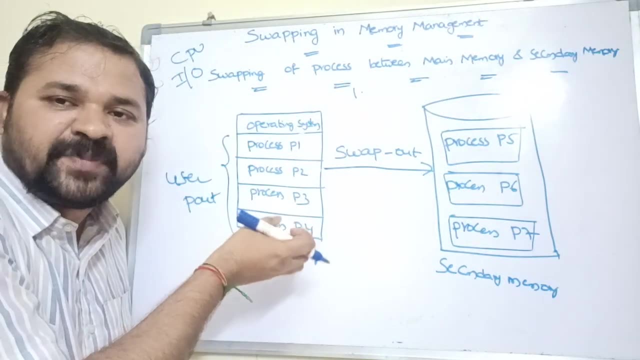 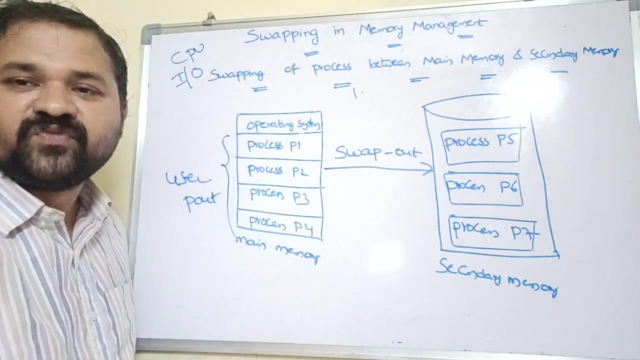 operating system transfers a process from main memory to the secondary memory. this is the first scenario. so what is the first scenario? if a process completes its execution, then operating system transfers that process from main memory to the secondary memory. why? because the size of the main memory is. 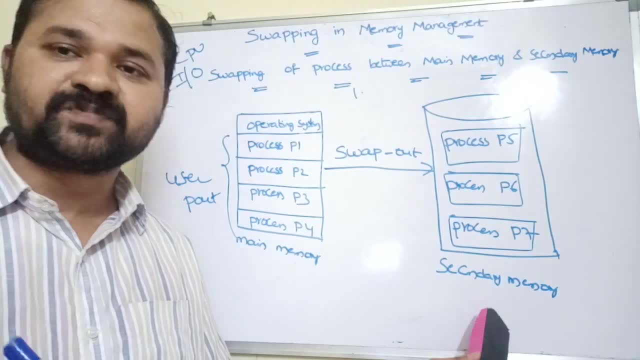 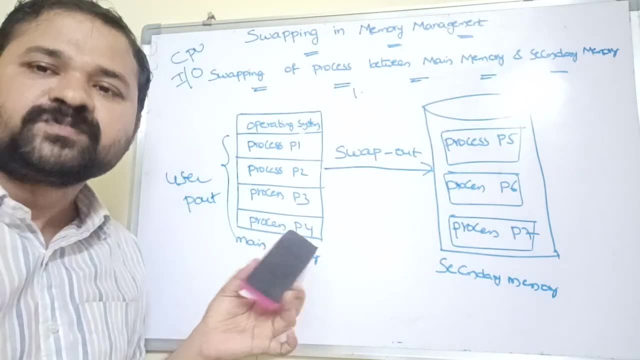 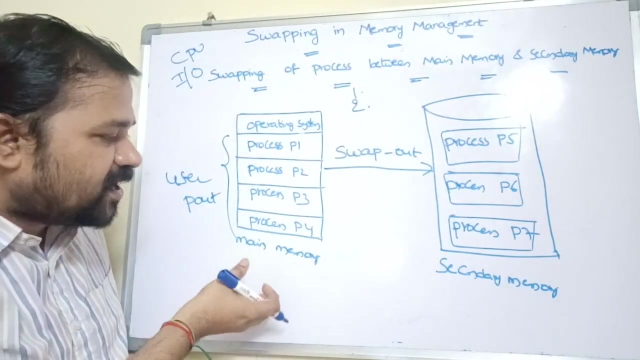 very, very small when compared with secondary memory. so p1 completes all its operations, so we can not store some other process in the main memory so that CPU can execute that process. let us take in this scenario where the transferring should be done from main memory into the secondary. 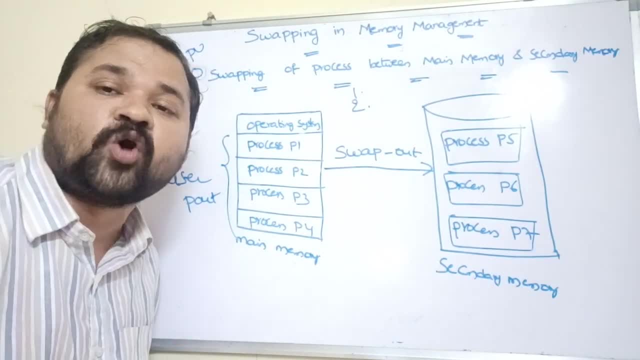 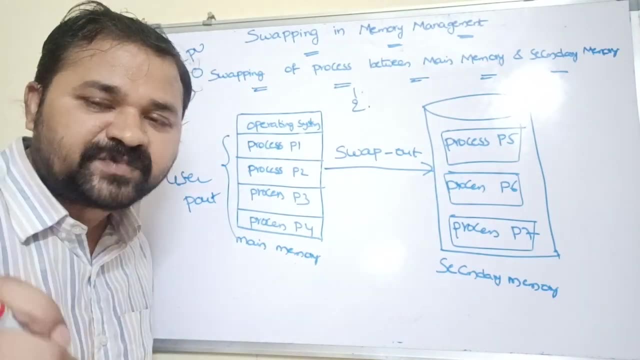 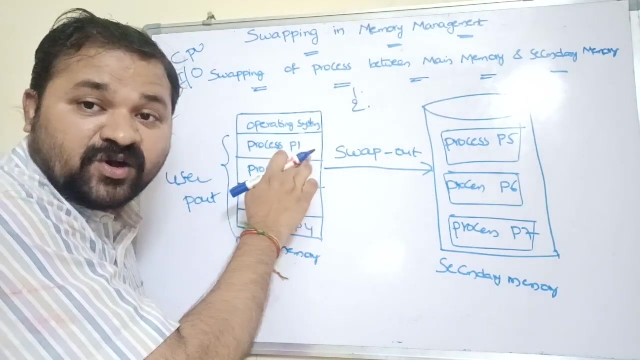 memory. let process p1 is waiting for some. I ghosts. let process p1 is waiting for some. I know operation, so during that time CPU is one id, so there is no need of cpu for process p1. why? because it is waiting for some ibo operations. 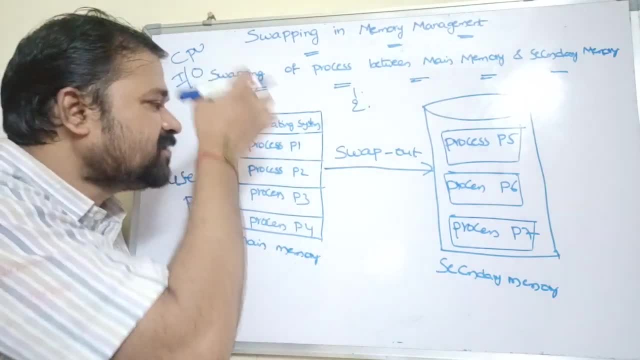 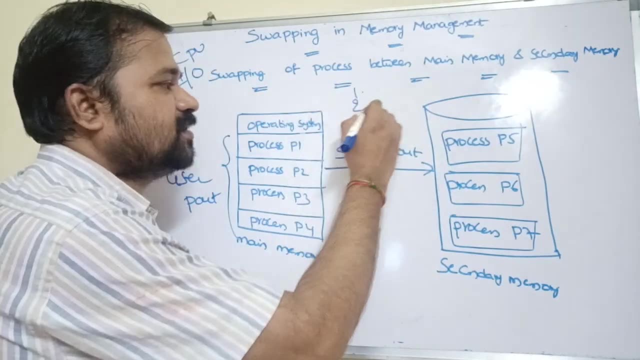 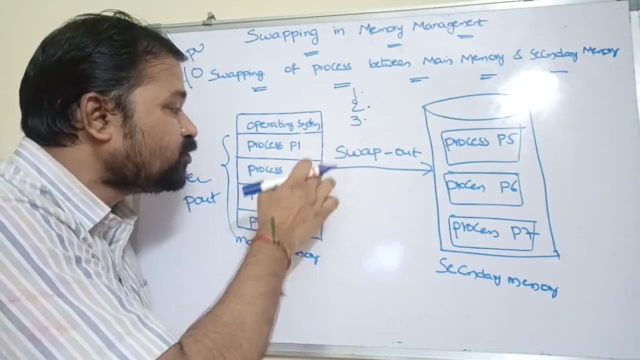 so what the operating system will do. operating system will transfers p1 from main memory to the secondary memory and this is known as swap out. so this is the second scenario. let us take the third scenario. let us assume that process p1 is trying to access some operating system area or 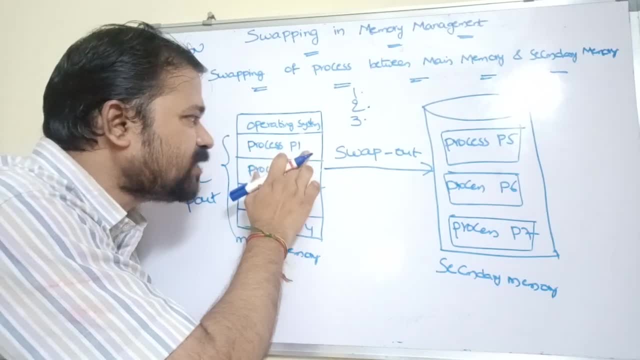 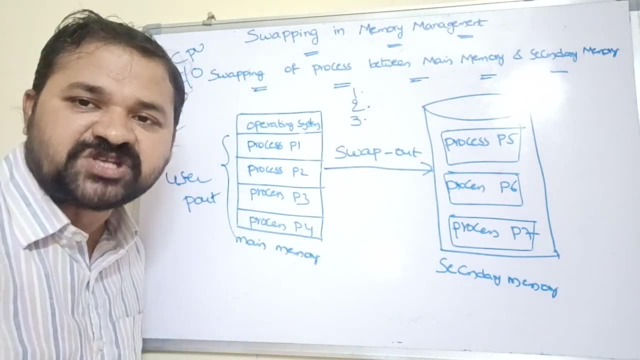 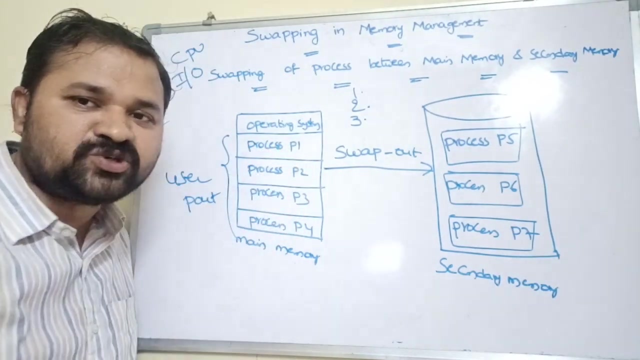 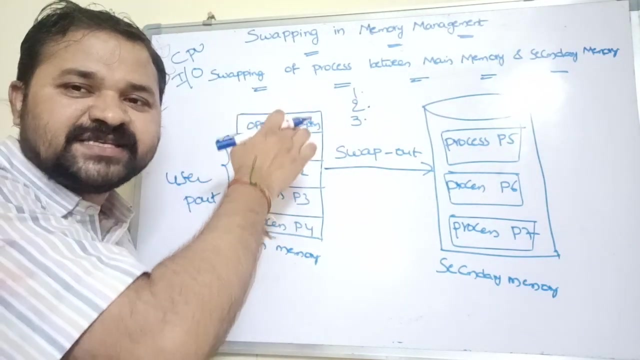 some other processes. let: process p1 is trying to access operating system or other processes, so some protection violation will occur. so operating system will generates a trap or interrupt. so this process execution, the process p1 execution, should be terminated. why? because it is trying to access other process area here. operating system can access any process, but 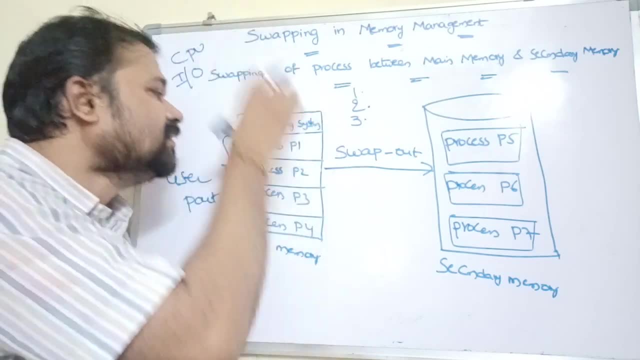 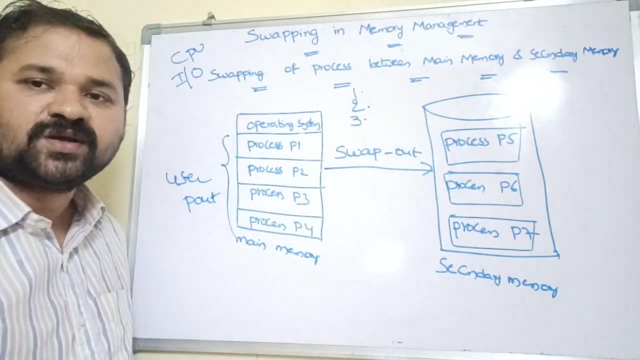 the corresponding process needs to access the operating system area or some other processes. let us assume that process p1 is trying to access only those instructions only. so p1 should not access p2, p3, p4. p2 should not access p1, p3, p4. 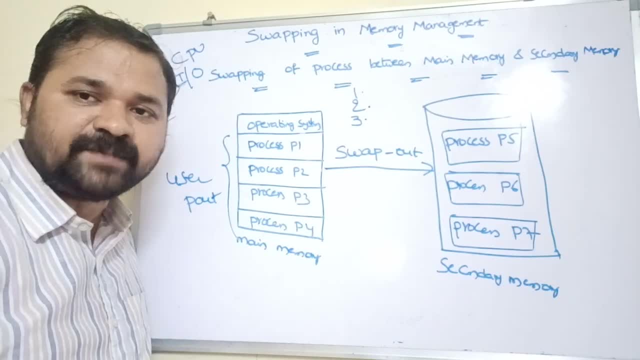 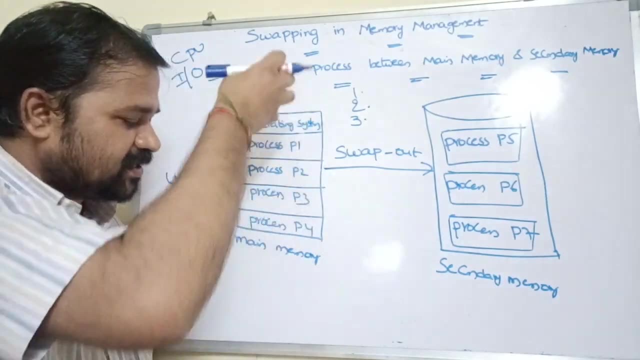 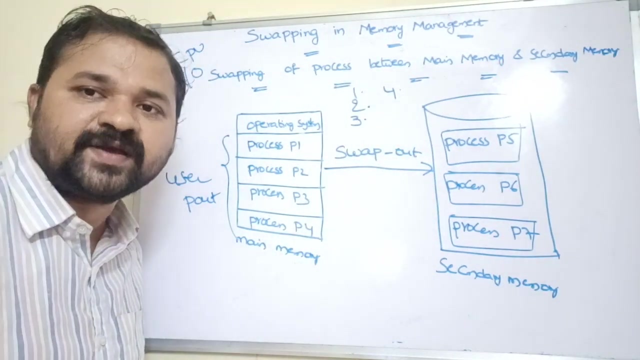 so in this situation it is trying to access other area so that operating system generates a trap, so this process will be terminated, so that terminated process will be moved from main memory to the secondary memory. so this is the tar scenario. let us take a round robin algorithm. 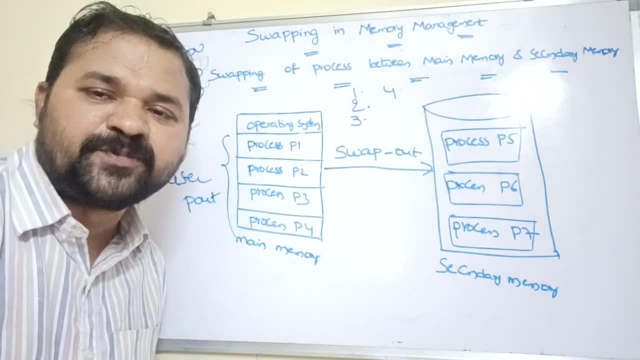 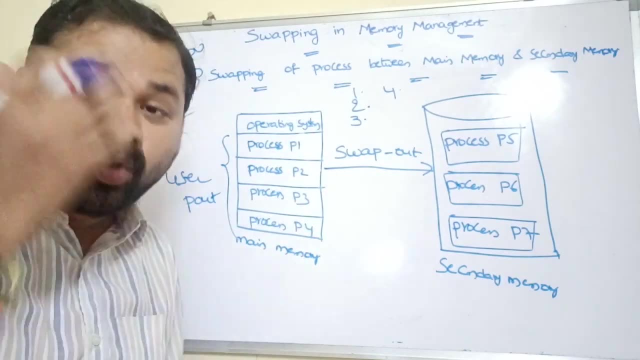 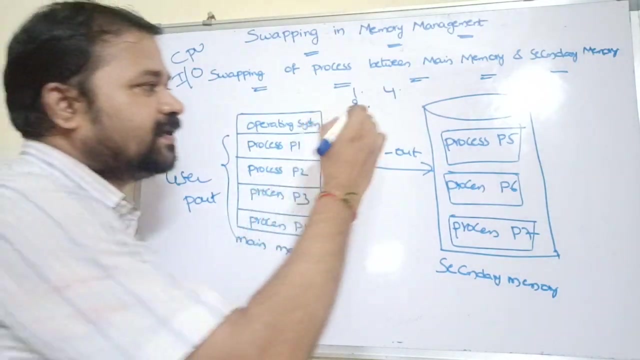 we know that in a round robin algorithm we execute a process for a particular time, quantum suppose. if that time quantum is completed, then there is no need of cpu for that process. so cpu transfers that process from main memory to the secondary memory. if you take priority scheduling algorithm, let us assume that process p1 is. 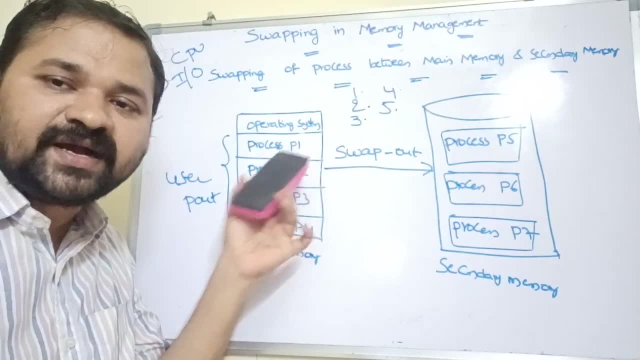 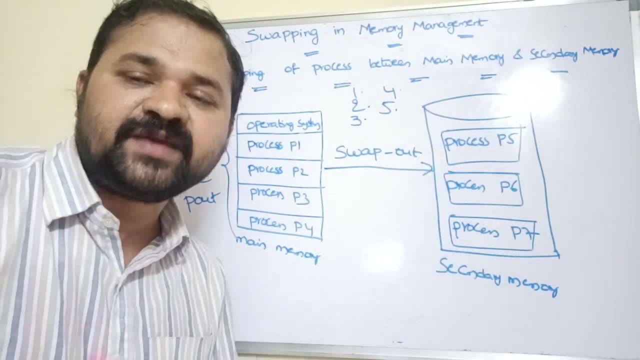 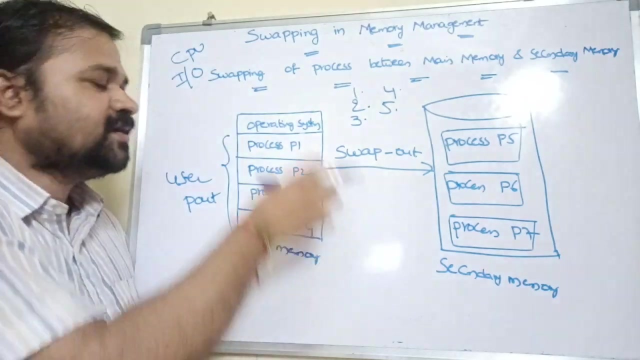 a low priority process. so while executing this p1 process, a high priority process came into the ready queue came into the secondary memory. so during the time also, the cpu has needs to stop the execution of process people. so this process p1 should be transferred from main memory to the secondary memory in order to execute what 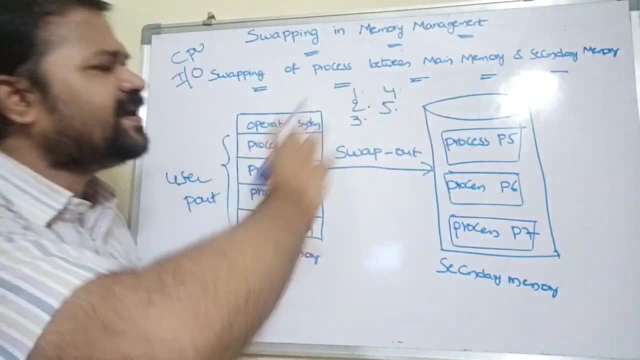 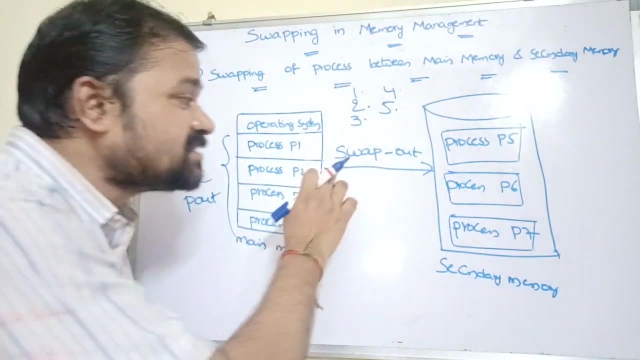 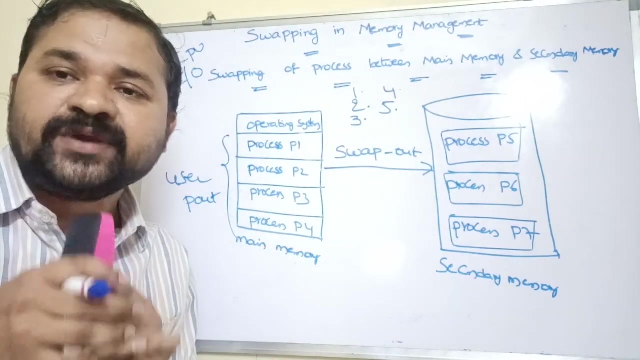 high priority process. so these are the various scenarios where a process will be transferred from main memory to the secondary memory and this transferring is known as swap out. and let. now the cpu is free, that means cpu is ready to execute a process. then a process will be transferred from. 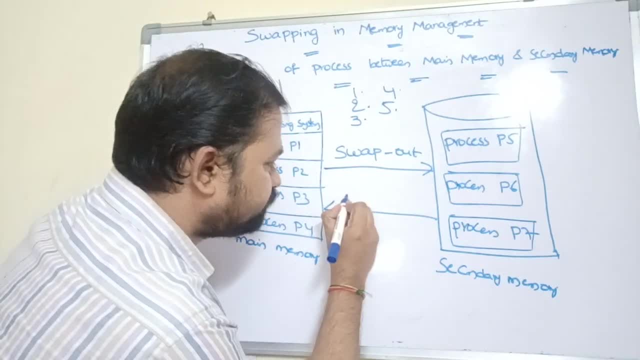 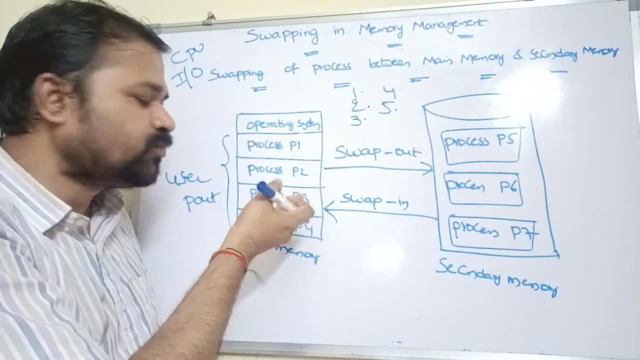 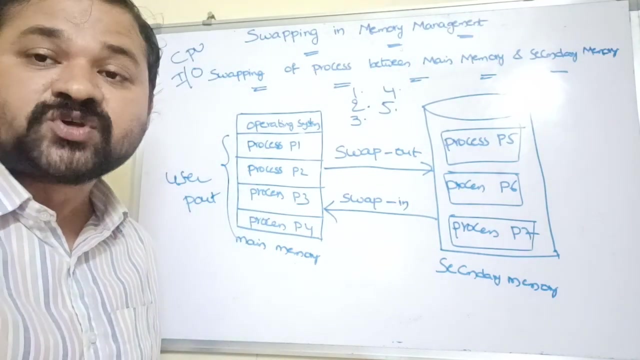 secondary memory to the main memory, and this transferring is known as swagging. let cpu completes process p1, process p2 and process p3 execution. let p4 is waiting for some ivo operations. so now the cpu is free. so what the operating system will do? operating system. 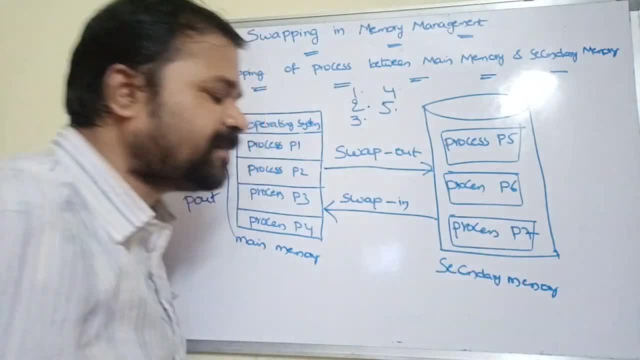 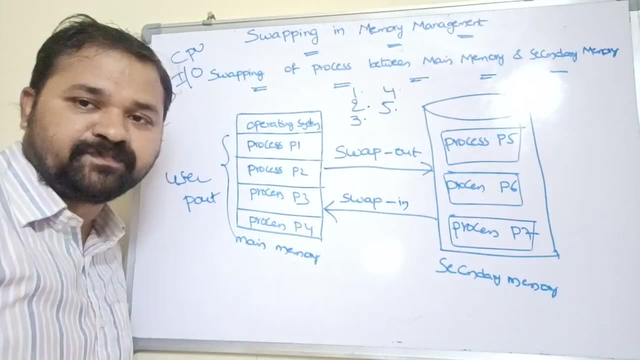 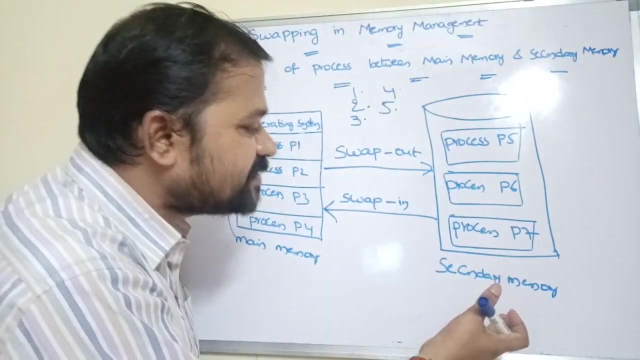 transfers a process. it may be p5 or p6 or p7. it transfers operating system, transfers a process from secondary memory to the main memory. why? because here cpu executes a process if it resides in main memory only. so transferring process from secondary memory to main memory is known as swap in. so this is about